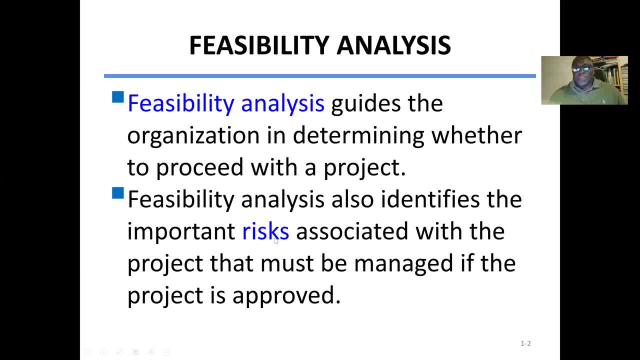 the project is approved, And feasibility analysis focus on three important aspects. One will be the economic feasibility: Is the funds available for the project Or the costs and benefits? This is good. And also technical feasibility: volunteerия verfée this technology. we want to use this. is it a new technology or has 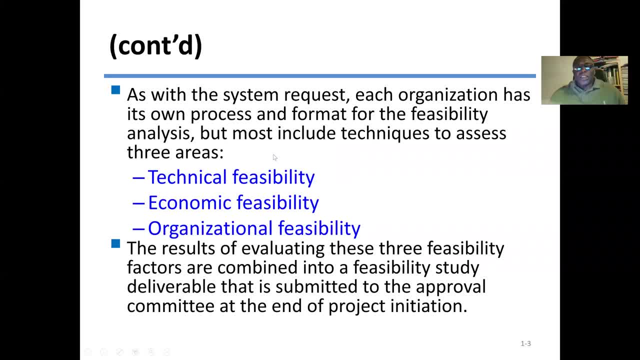 been used before. So here we say: as with the request, Each organization has its own process and format for the feasibility analysis, but must include techniques to assess the three areas: technical feasibility, Econcha Inc. Dynamic simulation feasibility, organizational feasibility. So the results of evaluating these three 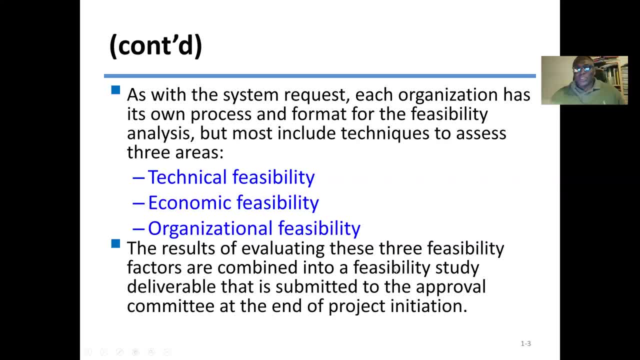 feasibility factors are combined into a feasibility studies, So technical feasibility is very important. Is the new project that we are going to implement? is it the new technology? If it's a new technology, the chance of failure of the project will be very high. If it's a whole technology which has been used, 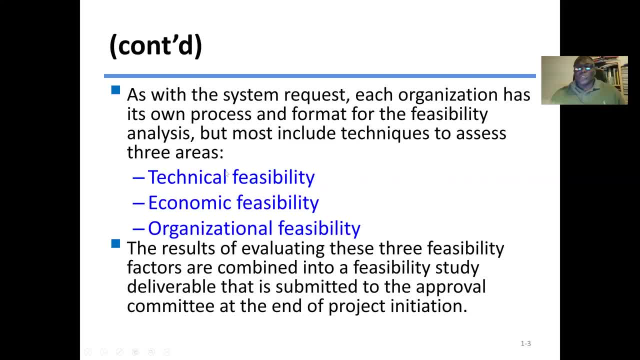 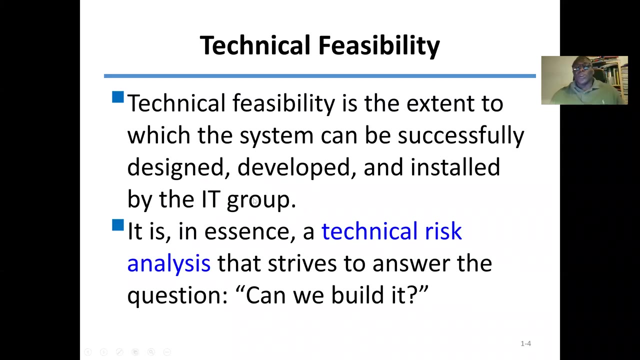 before. experience already taught us how the system will perform. So technical feasibility: if it's a new technology, we have issue of failure high. If it's a whole technology that has been used before, then success is very high, Failure is very low. Then also we discuss about organizational feasibility. So the first 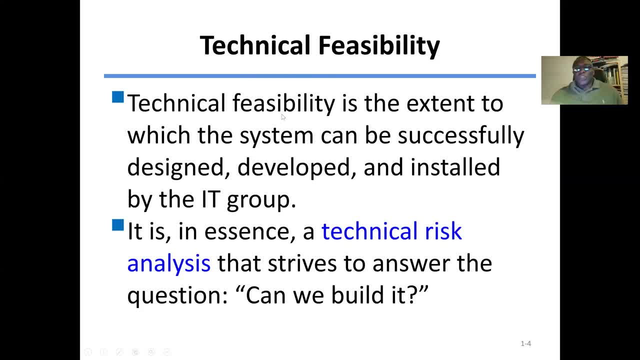 is the technical feasibility. Here we say technical feasibility is the extent to which the system can be successfully designed, developed, installed by the IT group. So we want to know if this technology for implementing the system is a new technology or it's an existing technology. If it's an existing, as we said earlier, the success, 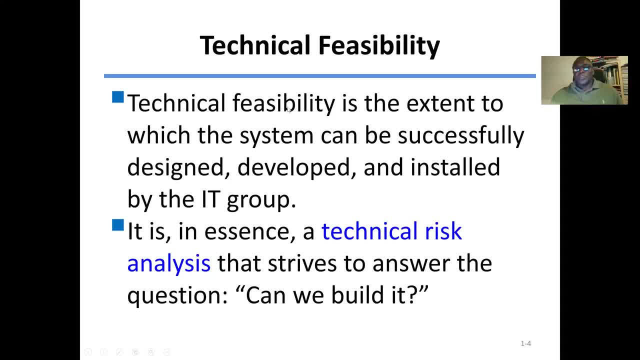 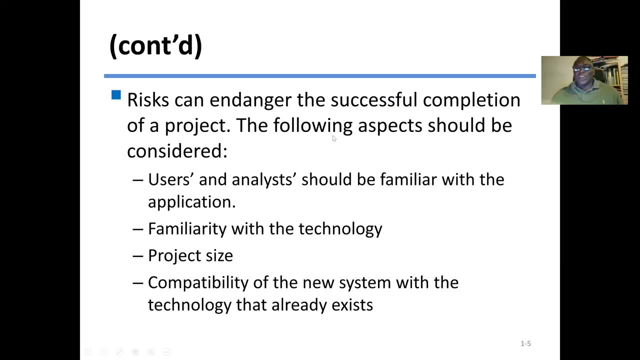 is very high. If it's a new technology, the chance of failure will be very high. So it is, in essence, a technical risk analysis that strive to answer the question: can we build a sphere of product? Risk also can endanger the successful. 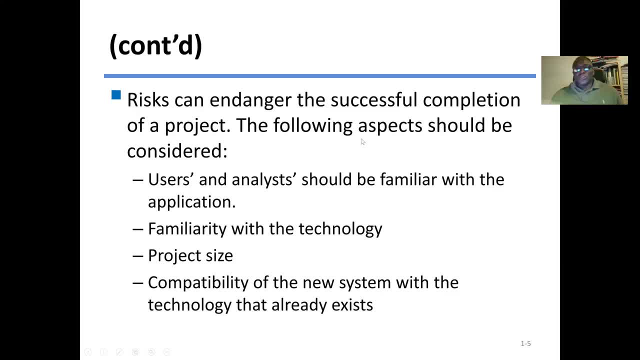 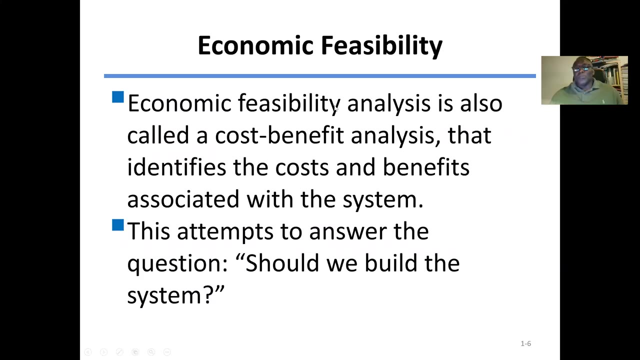 completion of a project And the following aspects should be considered: For example: the users, the analysis- should be familiar with the application or with the technology. Familiarity with the technology. project size now compatibility of the new system with the technology that already exists. Economic feasibility- here we are talking about the cost and 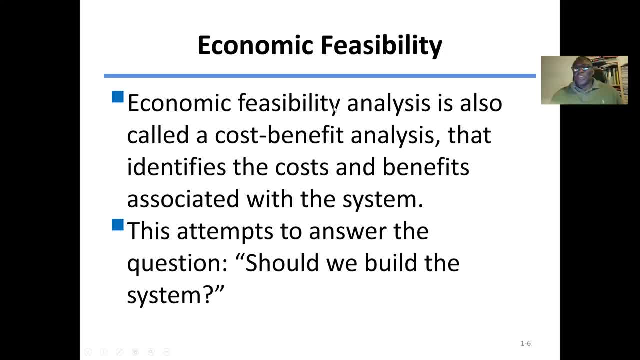 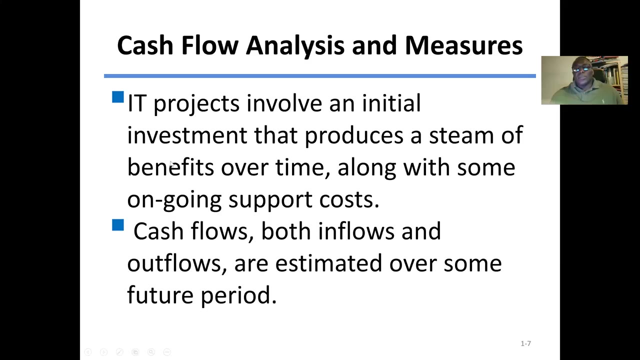 benefit of the system. So cost and benefit analysis: Is the cost outweighing the benefit, Then we don't need a system. But if the benefit, the cost is reduced and the benefits is high. So cash flow analysis and measures. The IT project again involve an initial investment that produces a stream of benefits over time. 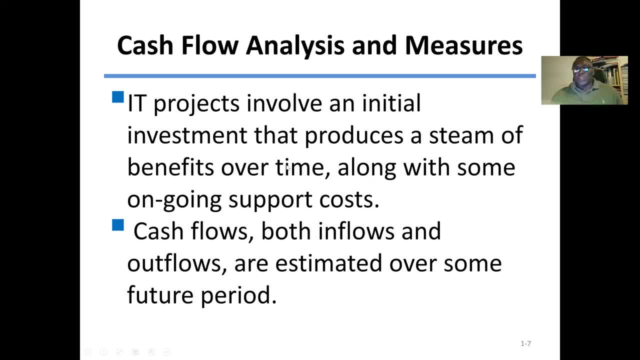 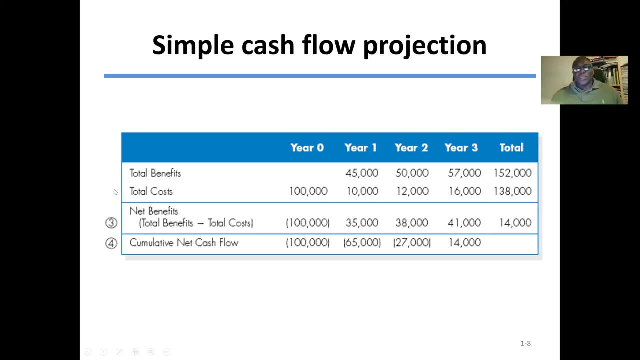 along with some ongoing support costs. So cash flow, both the inflow and outflow, are estimated over some future period. So this example is simple cash flow projection. Here we say we have a project And then the total benefit for years It's zero, it's nothing. By year one we say 45,000, year two 50,000, year three 57,000.. 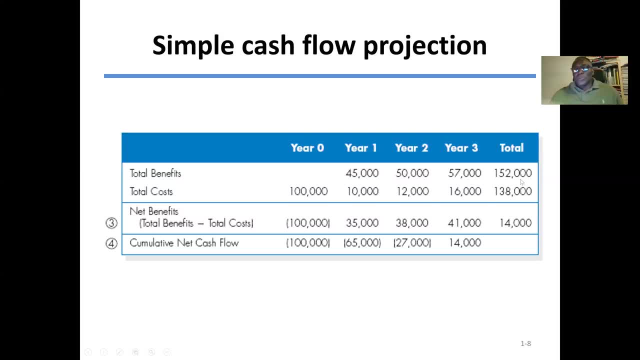 So in a total of three years the total benefit will be 152,000.. Total cost is 100,000, beginning then 10,000, 12,000, 16,000, total is 138,000.. So the net benefit here will be 14,000, which 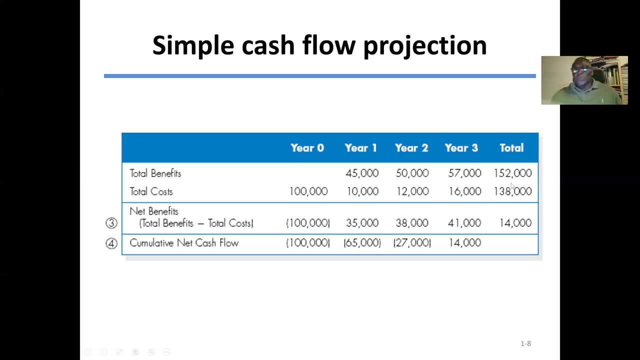 is 158,000 minus 138,000. The total benefit minus the total cost. Now, if the net benefit is 158,000, the total benefit minus the total cost. Now if the net benefit is a negative value, then it's not a good idea, which means the costs totally. 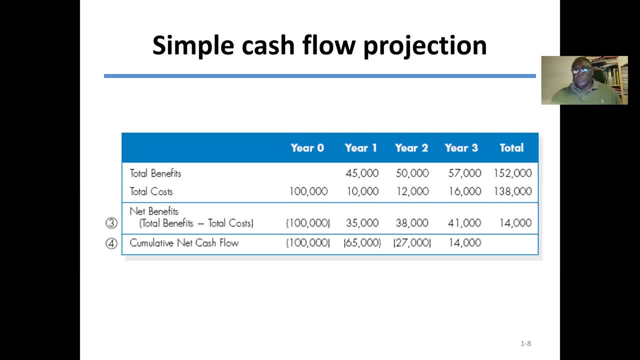 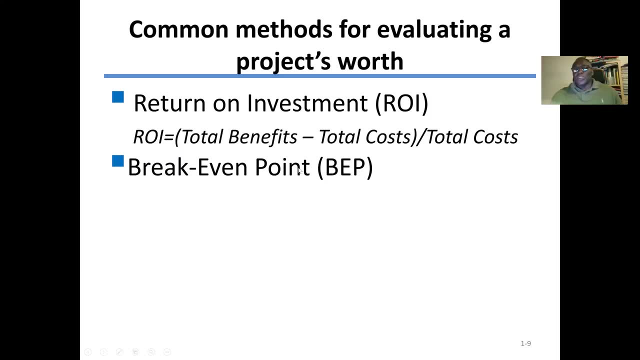 are to win, It's more than the benefits. So common methods for evaluating a project worth we can use the return on investment. So return on investment would be the total benefit minus the total cost divided by the total cost, Also break-even point. 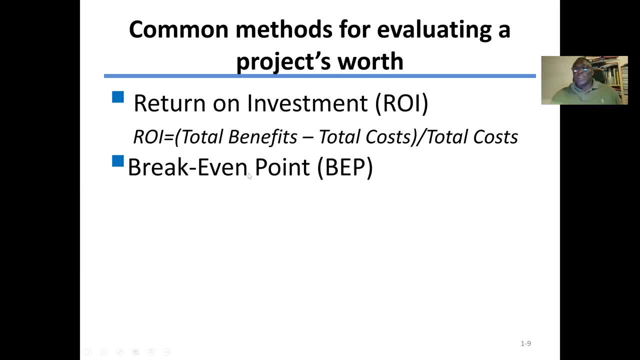 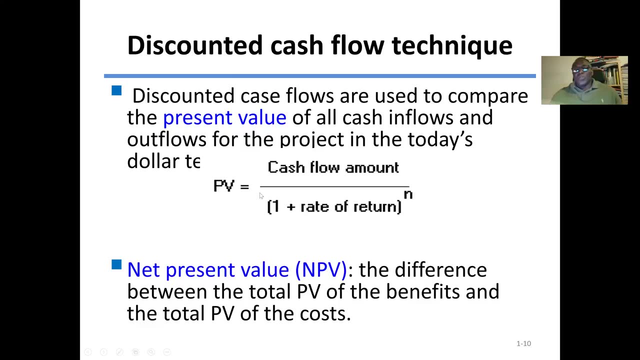 Where the total cost, The total cost and the total revenue are the same, We can analyze the break-even point. So this is an example of a break-even point. So discounted cash flow techniques- Here we said discounted case flows- are used to compare. 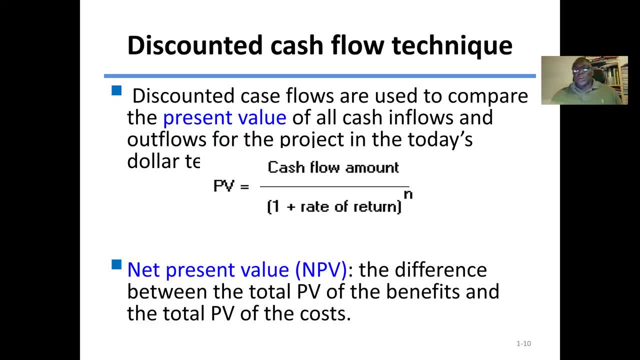 the present value of all cash inflows and also add flows for the project In today's dollar. Okay, So the P V, which is the present value, obviously, is the cash flow amount divided by one plus the rate of return to the power N, and would be the number of years or the period Also. 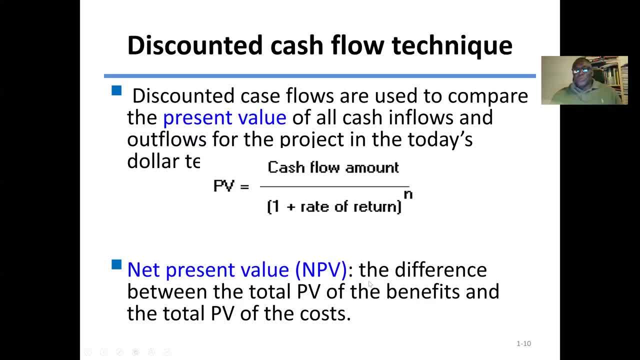 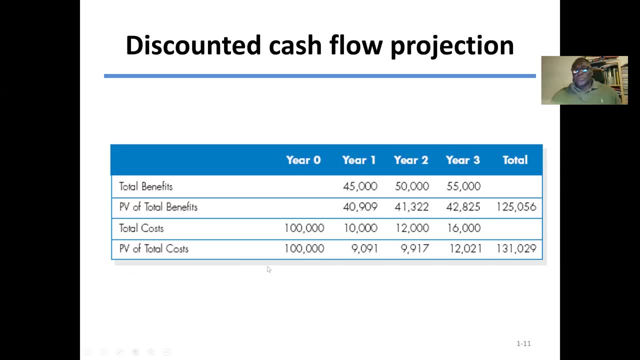 we said, the net present value is the difference between the total present value of the benefit and what the total present value of the cost, And that will give us the next, the net present value of the total benefit. So this example, again we can see: the total benefits, the present value of the total benefits. 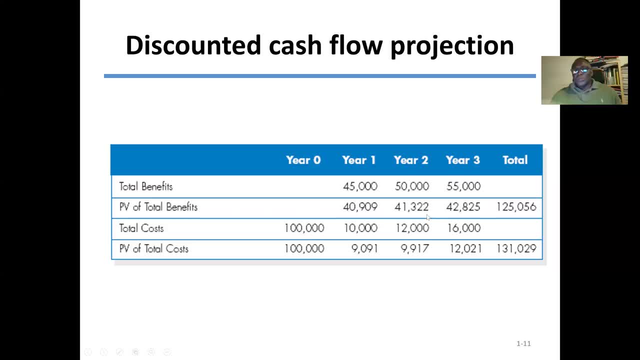 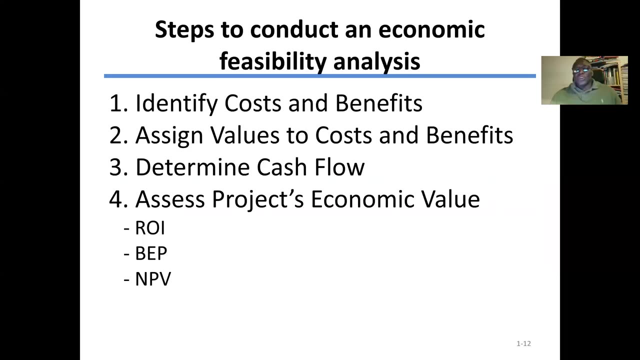 Then we have total costs and the present value of total costs. So steps to conduct an economic facility. Okay, We're still going to identify costs and benefits. So here we have the cost and benefit. So we'll look at the cost and benefit analysis. 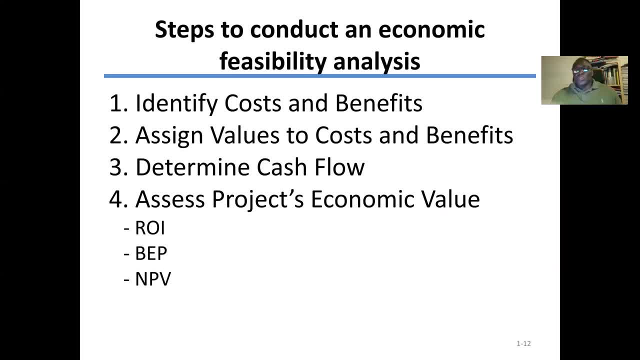 First we should identify the costs and benefit. Then we need to assign values to costs and also the benefit. Then we determine the cash flow. Then I assess the project's economic value- That's the example- whether it can be the minute return of investment or net present. 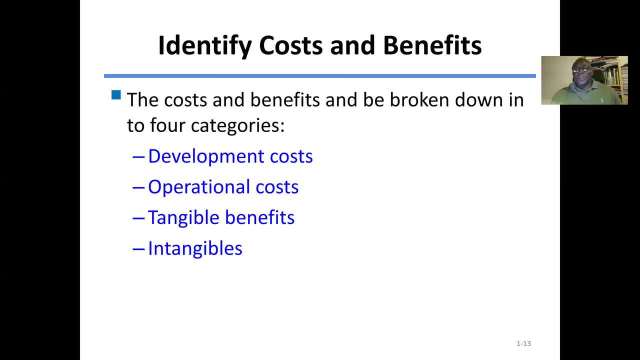 value calculations. So identify costs and benefits. Here we say the costs and benefits may be breaking down into five, four categories: the development costs, operational costs, tangible benefit and intangibles. an example give me. here we can see development costs, operational costs, tangible benefit and also intangible benefit. so intangible benefit can be. 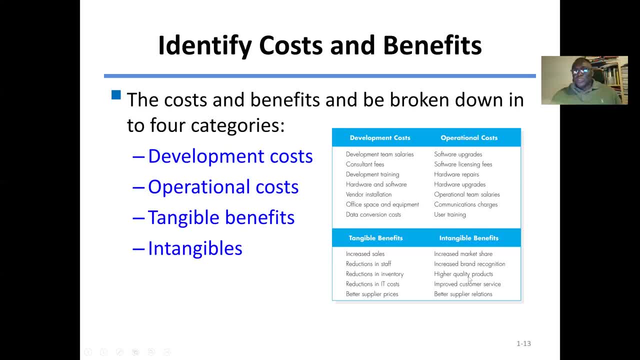 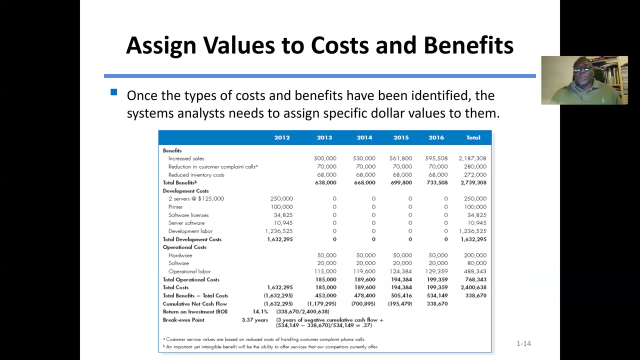 higher quality products. we cannot quantify it. reduction in inventory can be tangible benefit- we could, we can quantify it- or reduction in it costs. so this is an example given to where we assign values to cost and benefit. here we have the year from 2012 to 2016 in the total, so increment, increase, increase, sales. 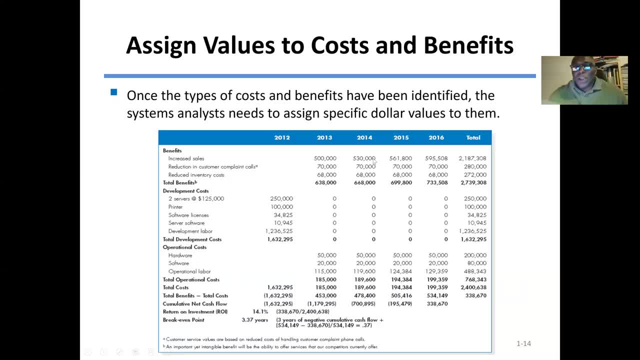 is for: yeah, we have half a million. by 2014 it become 530 000. 2015: 561. we can see that it's increasing. the reduction in customer complaint calls, and there was no any reduction. the same. reduce inventory costs: there was no reduction, it's the same. 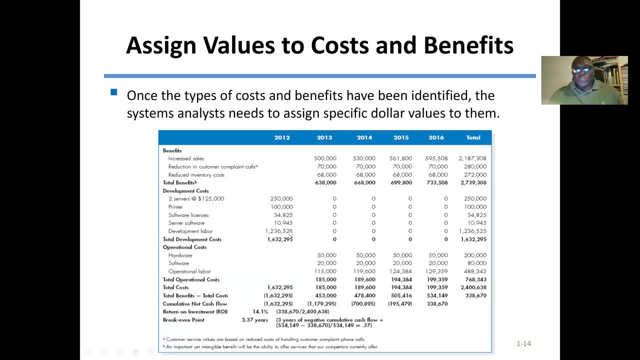 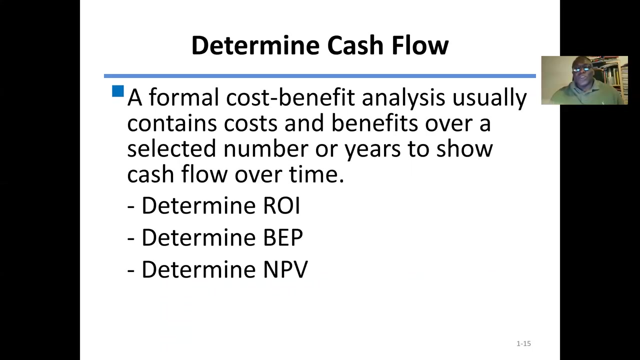 then we also have the development costs. in this case we said two, seven by two servers, a printer, software lenses, software server, software development labs. so determine the cash flow. here we say the former cost benefit analysis usually contains the cost and benefit over selected number or years to show cash flow over time. so we can determine the roi, which is the return of investment. 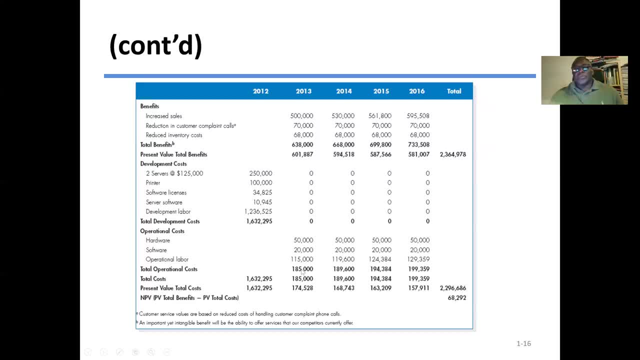 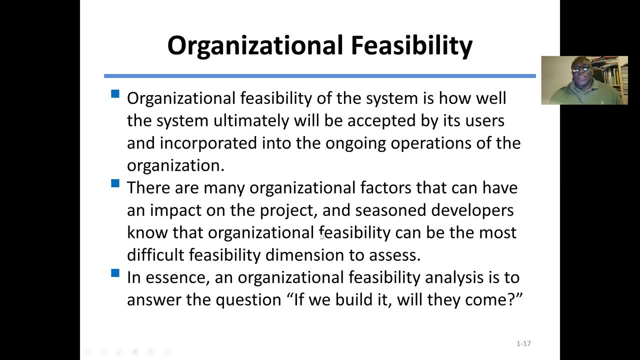 or be ep or mpv. so the next is the organization feasibility, and here we see organizational visibility of the system. it's how well The system automatically will be accepted by its users and also incorporated into the ongoing operation of the organization. There are many organization factors that can have an impact on the project and also seasoned developers. 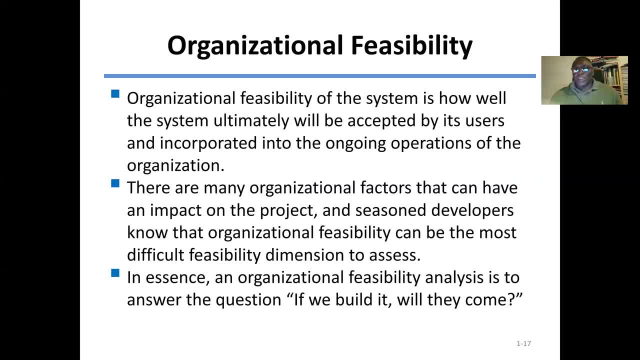 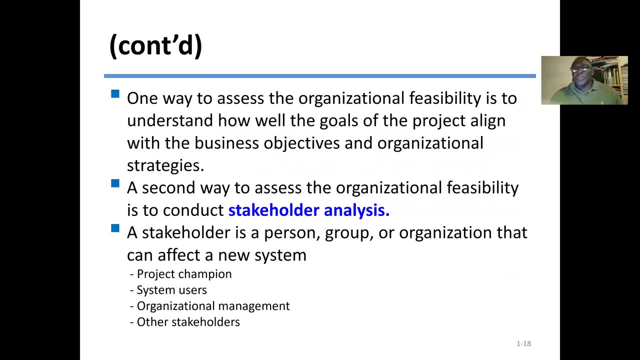 knowing that organization feasibility can be the most difficult feasibility dimension to assess And, in essence, an organization feasibility analysis is to answer the question: if we build it, will they come? Or one way to assess the organization feasibility is to understand how well the goals of the project align with the business objectives and organizational strategy.